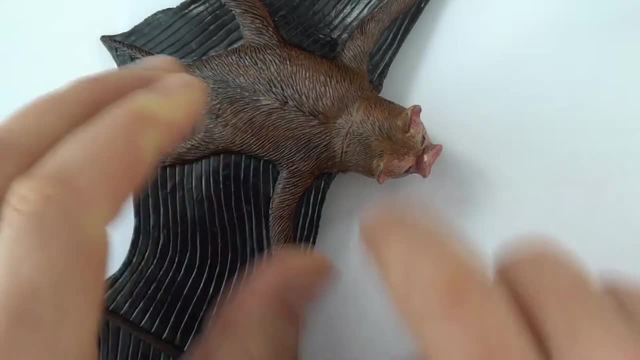 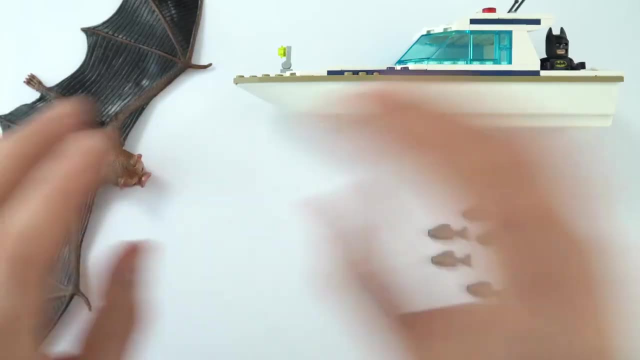 So how does a bat know how to find its prey when they're quite small and they're moving quite fast and it can't see them because it's nighttime? Or, equally, how does the boat know how deep the water is that it's floating in? Or maybe there's a fisherman and they want? 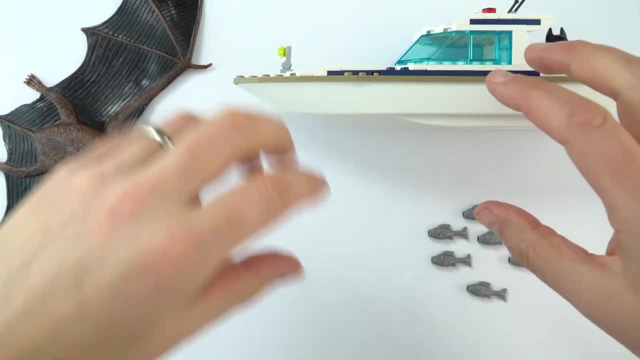 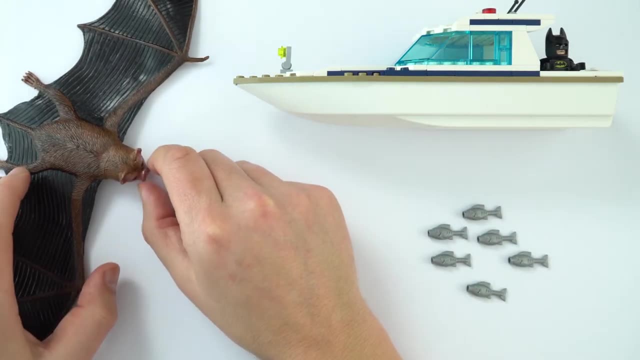 to find out where that shoal of fish is. How does it actually detect what's underneath it? Well, both of these things use this echo location. Now for a bat. it sends out a really high-pitched signal. above 20,000 hertz. It's actually out of the audible range of humans. 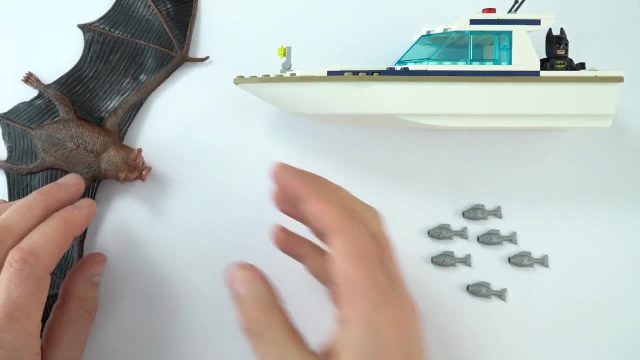 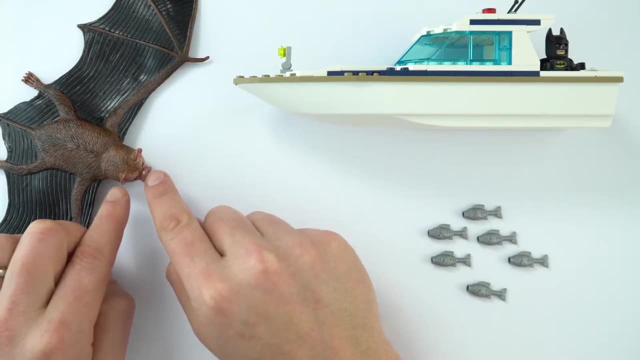 but it sends out this ultrasound signal, It comes away from the bat, it reflects off the prey and then some of that signal is bounced back And if the bat can detect how long it took for it to go there and come back again, it can then work out the distance We use. 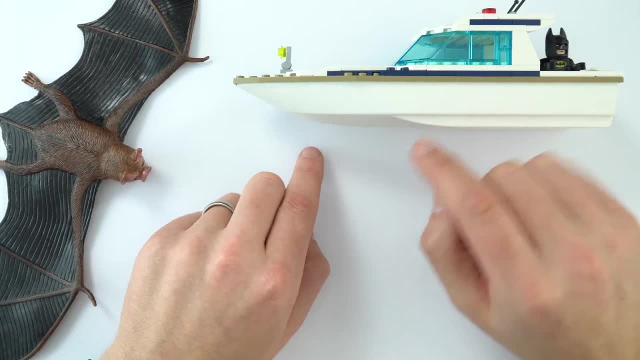 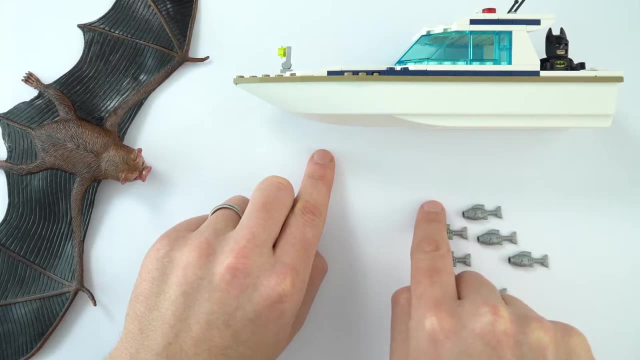 the same thing with sonar. So this is using audible sound, And what happens is that a signal is sent out from the boat. Some of that signal is bounced back, And then the signal is reflected off whatever it's looking for, And then the boat basically times how. 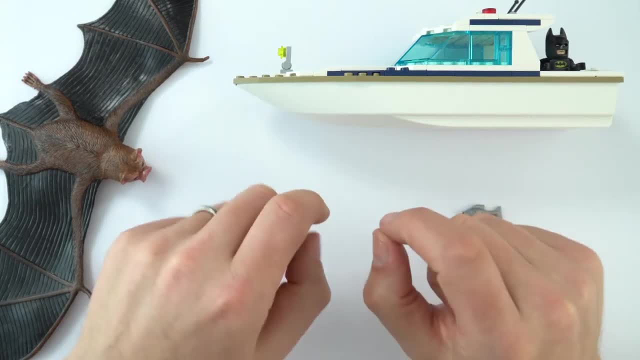 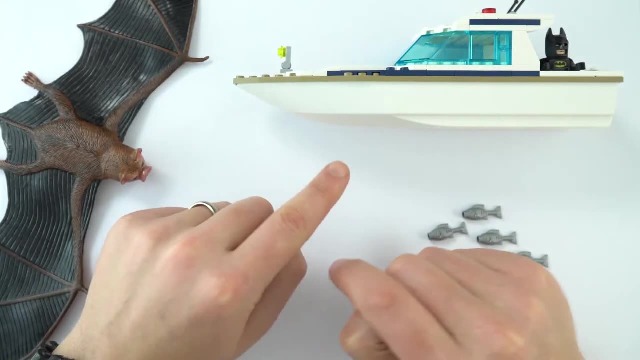 long it takes for the signal to go there and come back again. Now, if we know the speed of that wave in that medium- so maybe we know the speed of sound in water and we know the time it took- we can then calculate the distance to that object. 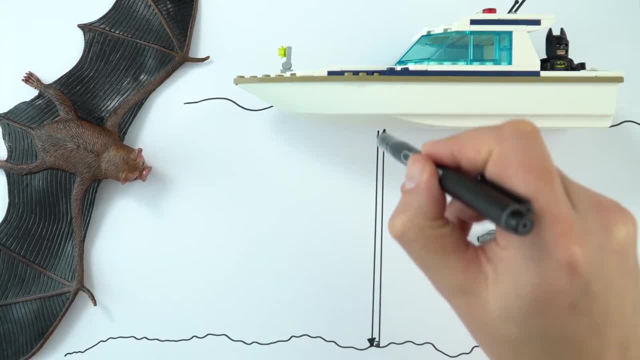 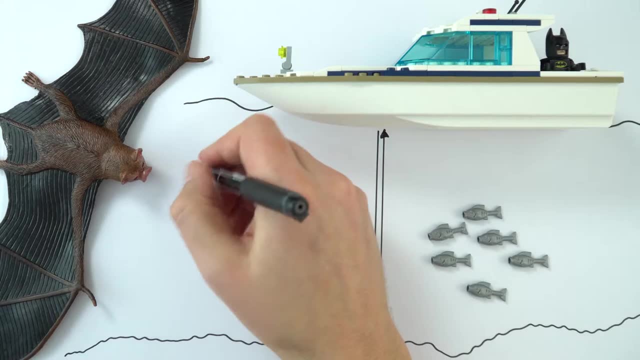 So we'll imagine there's a small unit down here. It sends out a signal. Some of that signal bounces off the bottom of the sea and then it was reflected back to the boat. Now what we might know is that we can actually record the time it takes for the signal to go from there to there. 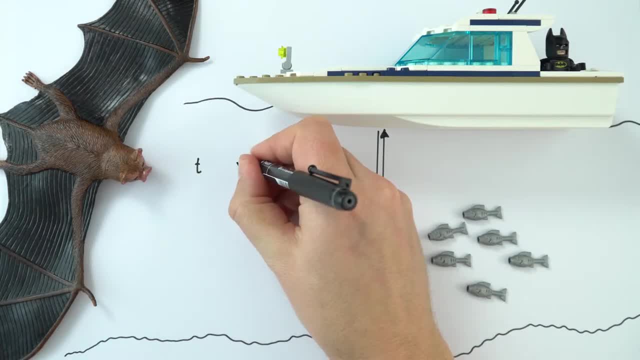 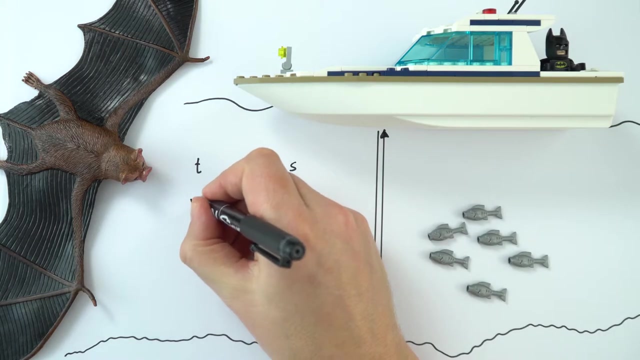 and back again. We might also know how quickly that sound travels in this sea water, for example, if this is a boat at sea, And we can then use this information to work out the distance above the bottom of the ocean. Now, here's the thing. We know that speed. 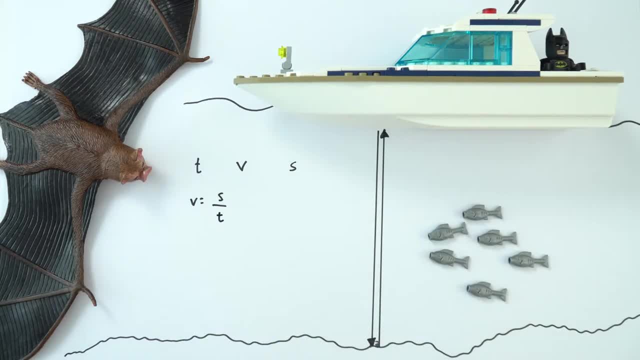 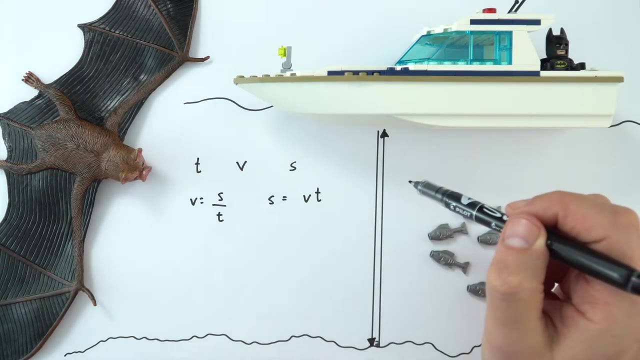 is equal to the displacement divided by the time, And therefore we can say that the displacement is equal to the speed times time. But if all we use is the time it takes to go there and back again, this is actually recording twice the distance that we need. So it's going there.